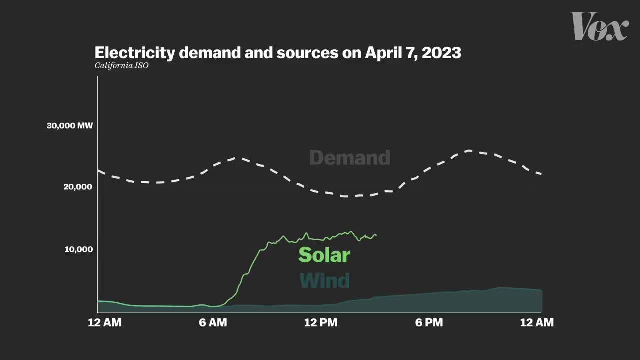 Solar panels, on the other hand, kick into gear around 7 am, generate a lot of electricity until the sun sets around 7 pm On most days. neither comes close to meeting the peak demands of the day, So the power company relies on fossil fuels like natural gas to make up for the gap. 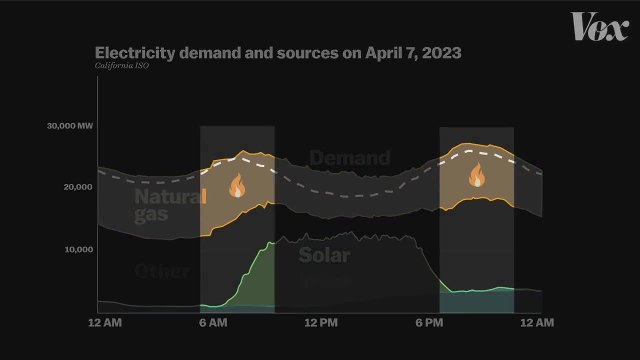 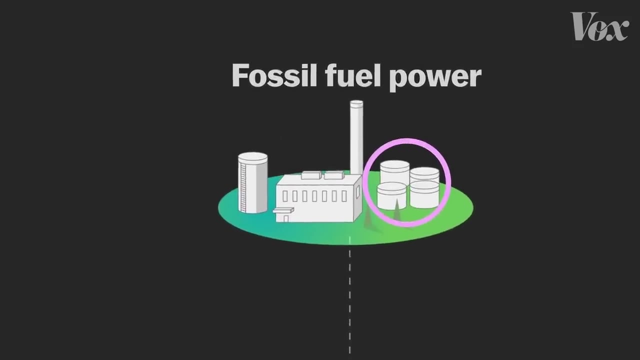 which widens significantly when people use electricity the most. Since the power company can't store the solar and wind energy, it has to use fossil fuels at these times, which can be stored in barrels and tanks. It's kind of the big gap in our renewable energy system right now. 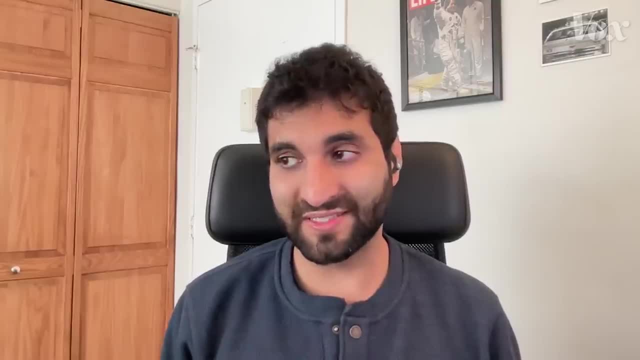 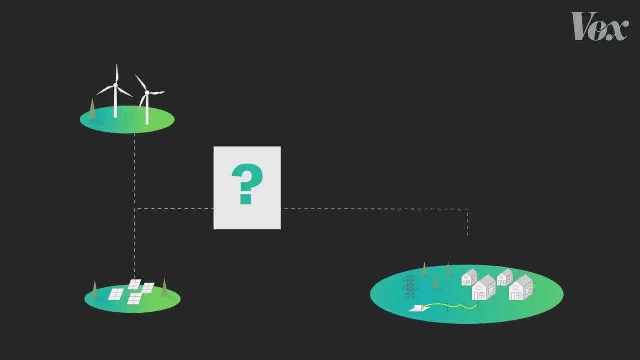 If we don't figure out a way to store renewable energy, there's a chance that we're going to be still dependent on fossil fuels. So how do we store some of this solar and wind energy? Well, we're going to have to figure out a way to store energy for later. 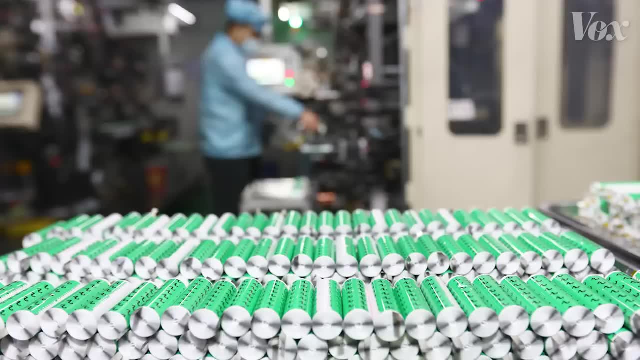 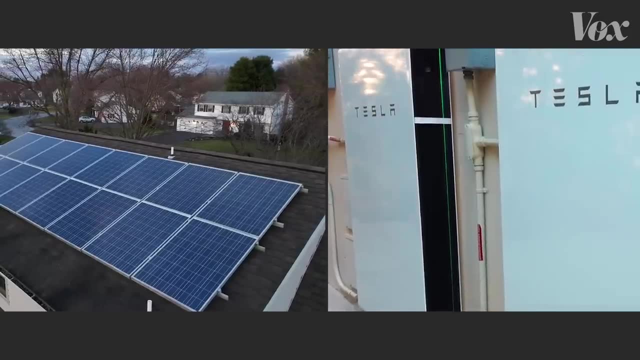 Right now you might be thinking: just use a battery, And you're not wrong. Batteries have improved immensely over the past few years, particularly lithium-ion batteries, which use a chemical reaction to store energy. Individual homes that have solar panels often use lithium-ion batteries to store energy. 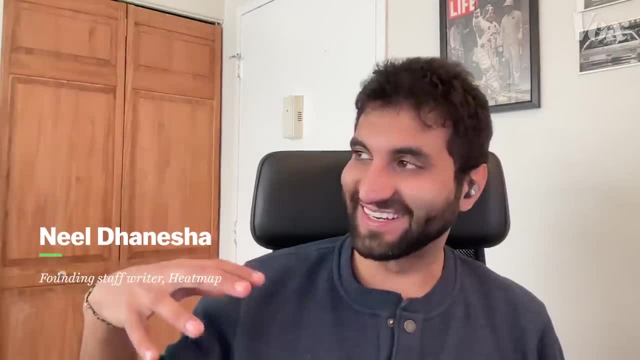 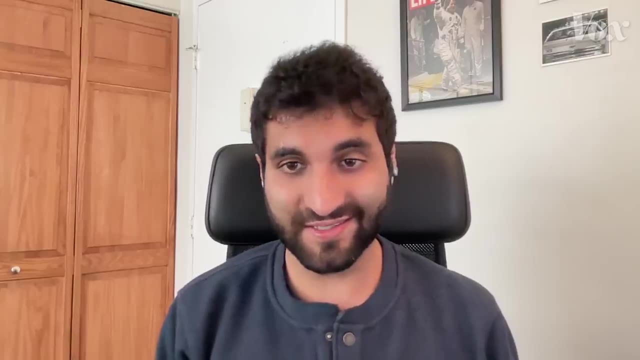 But there's a few reasons lithium-ion isn't perfect for the grid. This is Neil Dinesh, a founding writer at Heatmap, a climate news site, And he wrote about this for Vox in 2022.. One is just the scale that's needed. 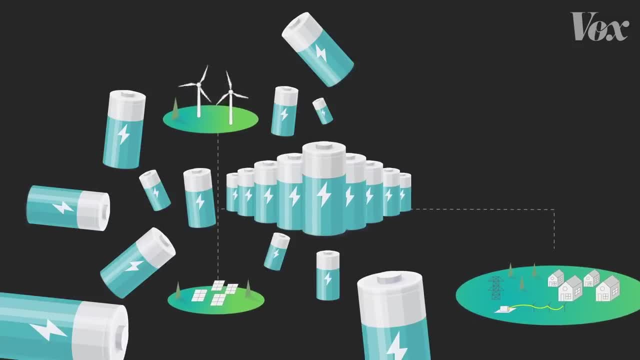 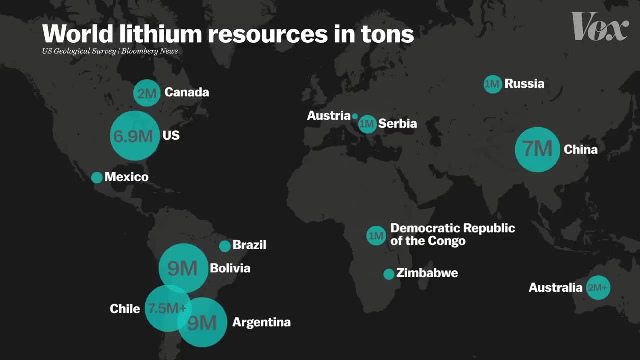 We would need a lot at a level that we just don't really have right now. That's a challenge, because lithium is only found in a few places on Earth, But, more importantly, like we need lithium-ion batteries for other things, Lithium-ion battery is really good for stuff that moves because it's relatively light. 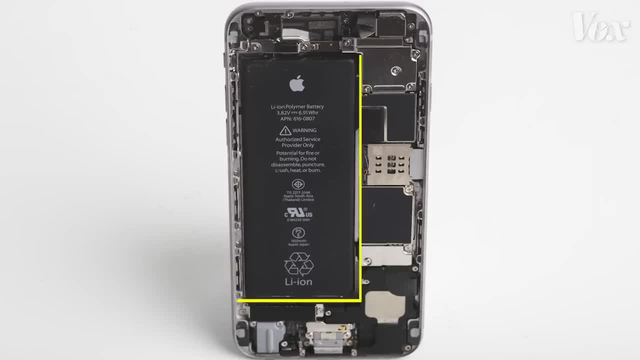 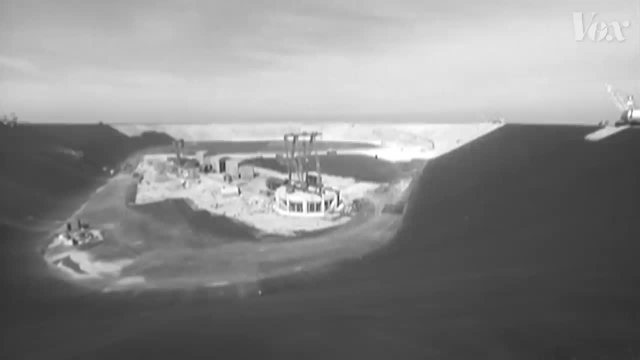 meaning it's better suited for things like electric cars and portable electronics, not power grids that stay still. Luckily, there's another energy storage solution that's actually been around for a long time. This is the site for the first power grid, The first pumped storage hydroelectric station in Southern Ireland. 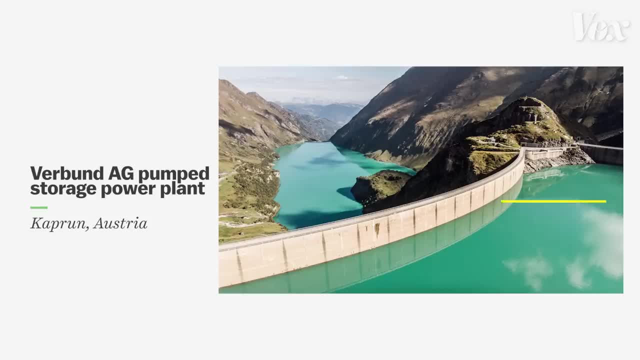 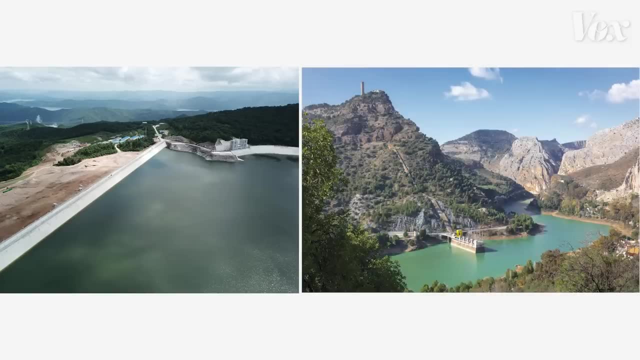 This is a type of energy storage called pumped storage hydro. They were first built in Europe. The US built one in 1929. And many more were built in the 1970s and 80s as a way to store nuclear power. 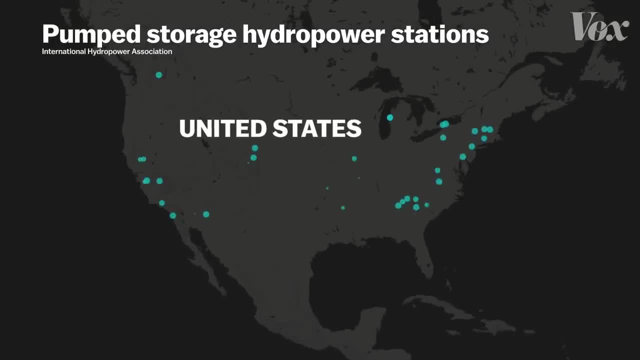 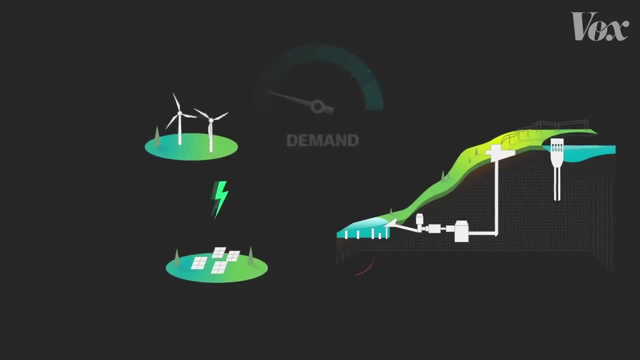 Today, these facilities are all over the world- There are 39 of them in the US- And they store energy in a really fascinating yet simple way. When energy demand is low, renewable or fossil fuel energy is used to pump water from a reservoir or river up a mountain. 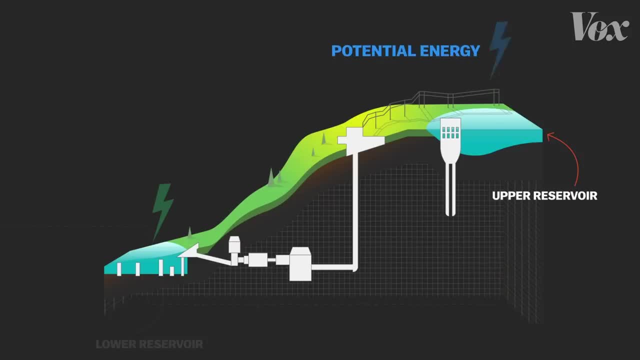 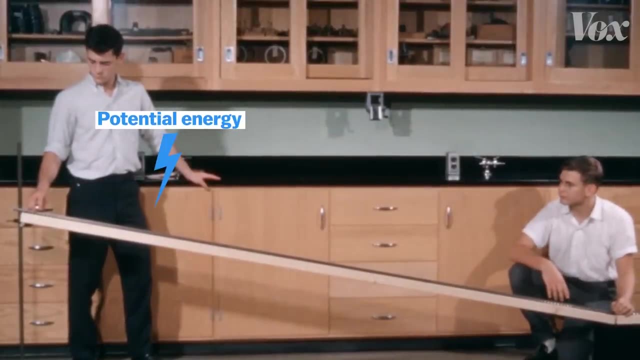 and then into a higher reservoir, basically converting this energy into what's called potential energy. So potential energy you might kind of remember from high school physics: When a thing is up at a height, it has stored potential energy. When it's let go, it turns into kinetic energy. 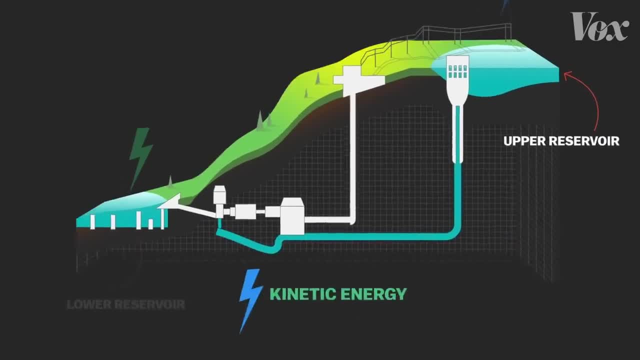 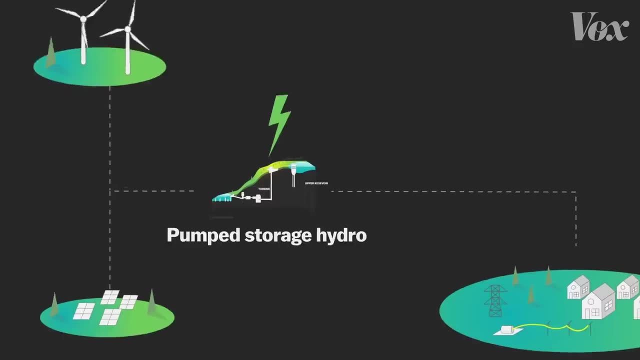 When that energy is needed. the water is released down the mountain, where it's converted into kinetic energy that spins a turbine and generates electricity for the grid. It's a way of combining water, a mountain and gravity into a battery, And it can be about 90% efficient. 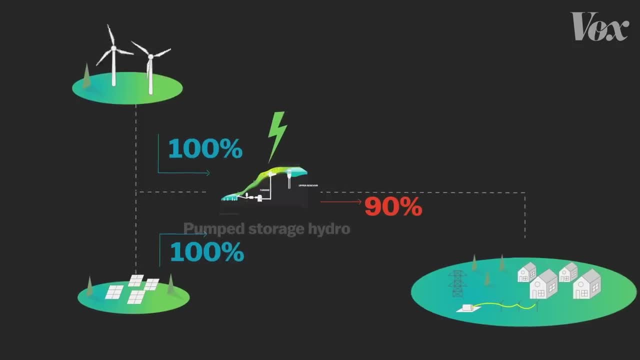 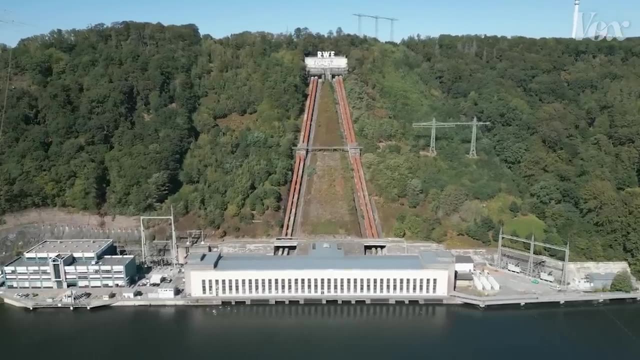 but only 10% of this energy is lost in the process. Pump storage hydro works really well, but it's difficult to build more Well. for starters, you need a mountain, And you need to haul out a mountain to put pumps inside it. 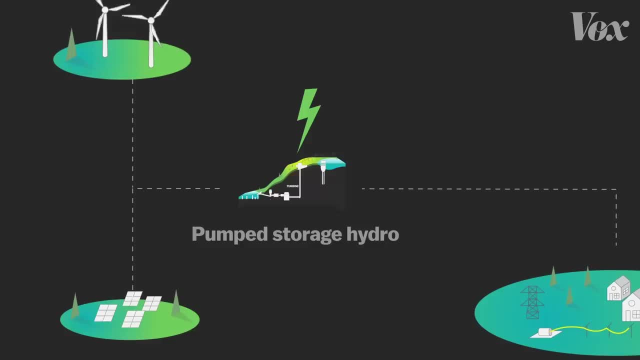 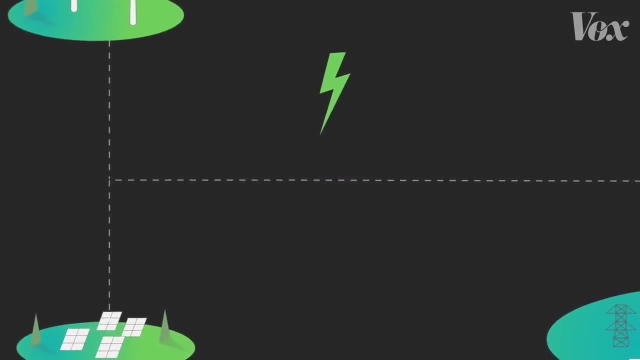 And it takes a lot of money, And we don't have mountains everywhere. So the ideal way to store renewable energy would be something that's cheaper and smaller than a pump storage hydro plant but works in roughly the same way. One company, Energy Vault, is also using gravity to store renewable energy. 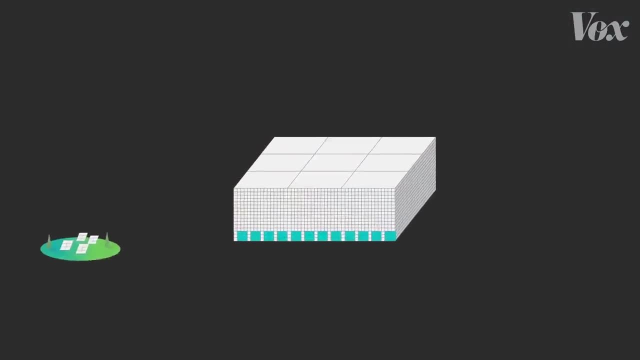 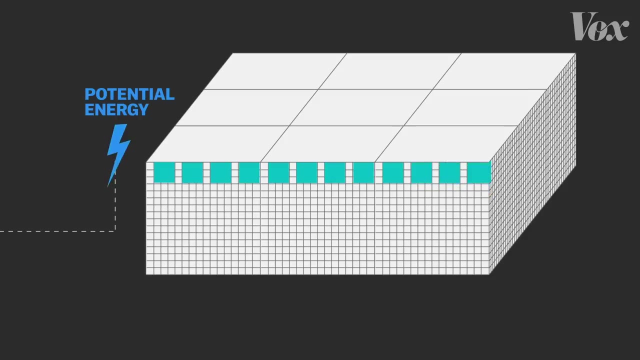 But without the water or mountain. Instead, renewable energy is used to lift heavy blocks of concrete up into the air, where it becomes potential energy. Then, when it's needed, the blocks are released, spinning a turbine which converts the potential energy back into electricity. 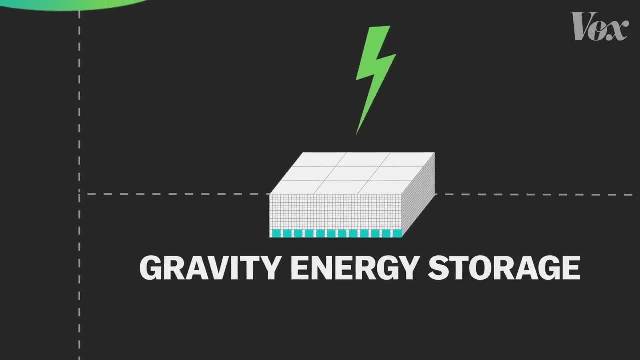 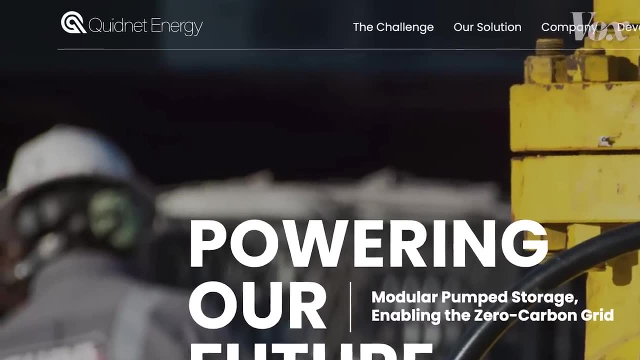 Energy Vault calls this gravity energy storage And, while it's still being tested, the company claims it could be more than 80% efficient. A company called Quidnet is working on a different version of the same principle. A mechanical pump storage unit uses renewable energy to pump water underground. 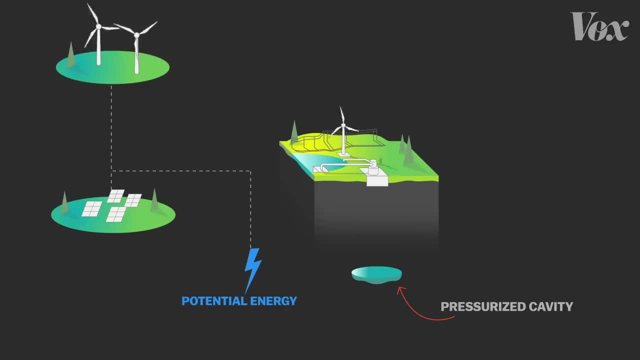 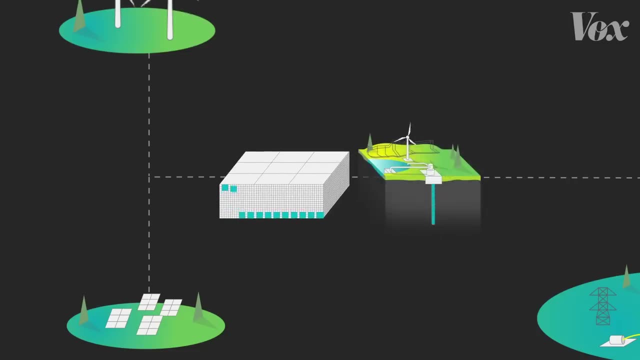 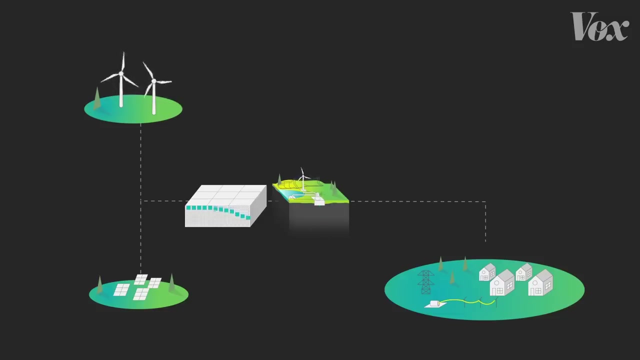 into a pressurized hole where it can be stored as potential energy, then released back up to the surface to spin a turbine and generate electricity. Both techniques are betting on potential energy as a solution for storing renewable energy for the grid. I think this is partly because potential energy has shown itself to be pretty efficient. Also realistically fewer moving parts. If all you're doing, basically, is using gravity to work with you, you have a pretty massive force of nature on your side right there. But potential energy isn't the only possible solution. Other companies are using renewable energy to superheat salt.